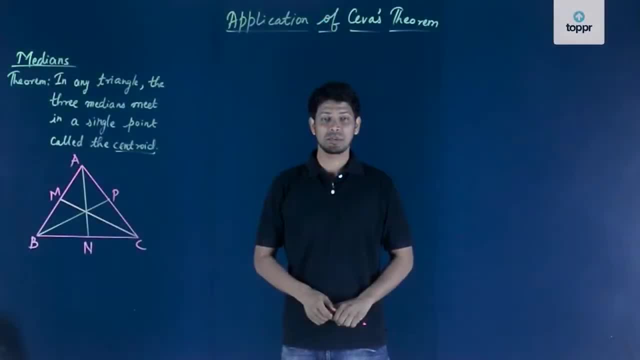 Hi students, today's topic of discussion is application of Siva's theorem. So here we will see one of the application that is median. So here the theorem says: in any triangle the three medians meet at a single point and that is called centroid. 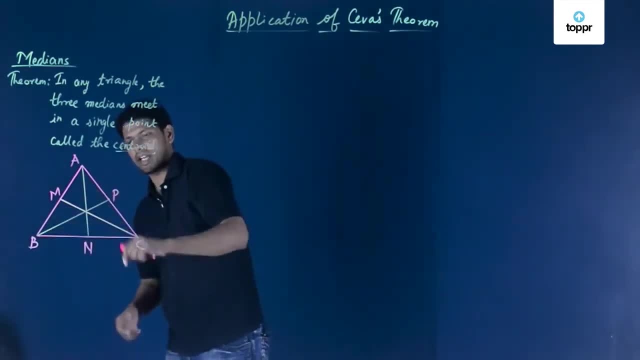 So see, this is a triangle: ABC and M is the midpoint of AB. okay, So AM is equal to MB and N is the midpoint of BC. So BN is equal to NC and P is the midpoint of AC. Therefore AP is equal to PC, okay, So. 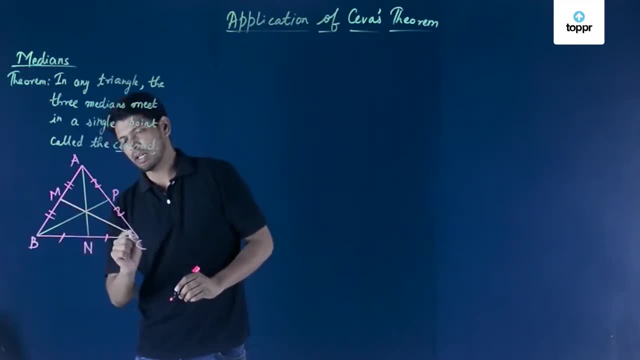 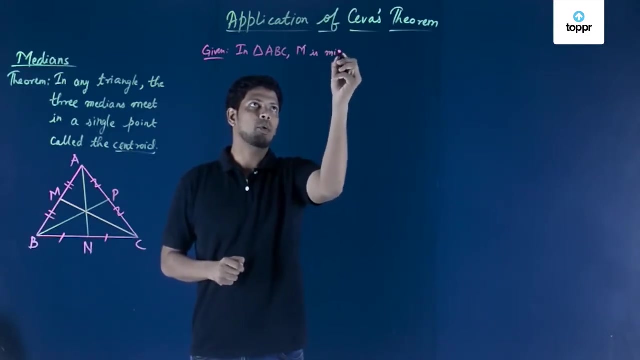 here. when we joined C and M, then it is the median, okay, and when we joined B and P, that is median, and when we joined ANN, that is median. So we have been given that in triangle ABC, M is midpoint, okay, of AB, okay, and N is midpoint of BC and P is 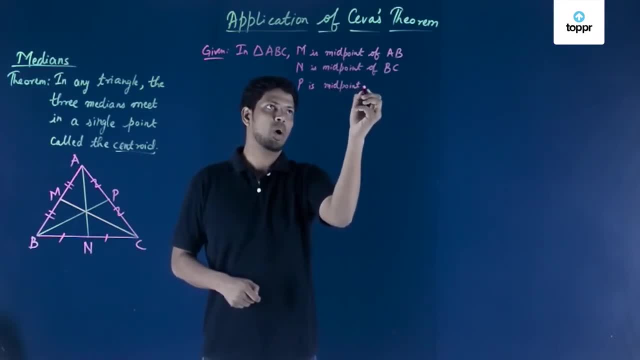 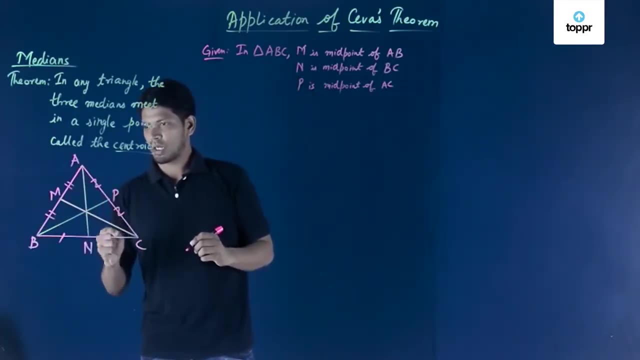 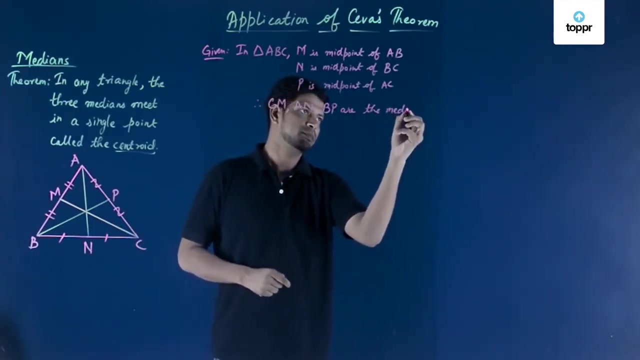 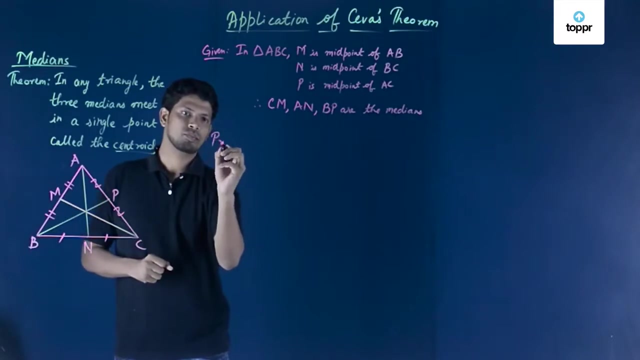 midpoint of AC. Hence we can say CM, okay, and AN and BP are the medians. So therefore, CM and AN and BP are the medians, Okay. so now let us see the proof. Ok, so we need to prove that, that the medians of AB are the equal of MC. For that answer, we need to find out which is median, which is F, okay, So now let us see the proof. 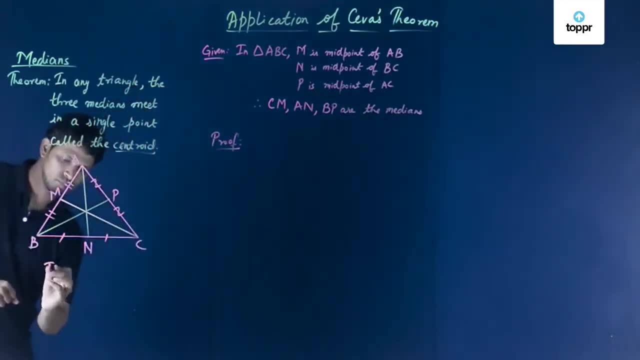 we need to prove that, since these are three medians, they should meet at a single point. We have to prove that medians of triangle meet at a single point. So this is our to prove. okay, So now with this, we know that M is the mid. 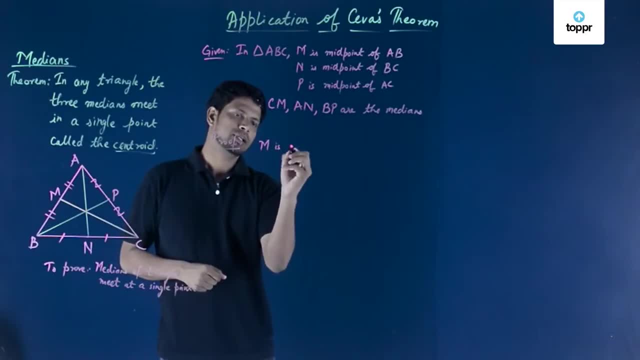 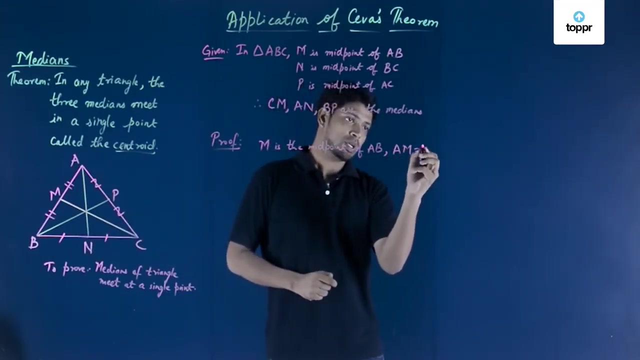 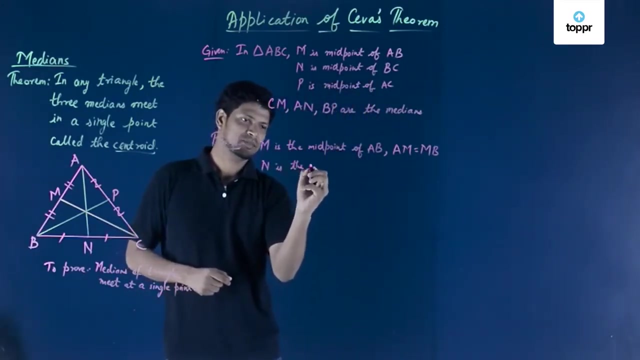 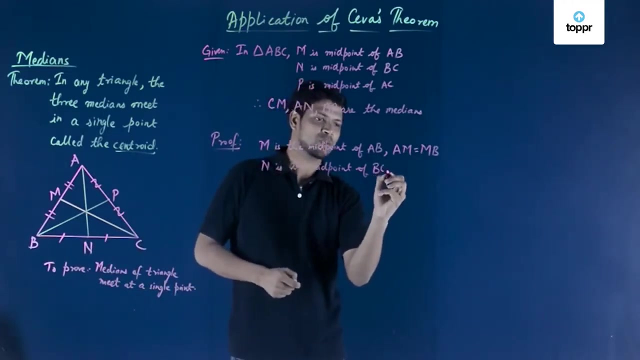 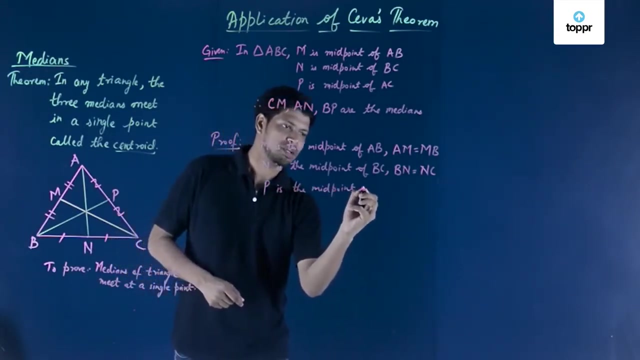 point M is the midpoint of side AB, So we can say AM is equal to MB, AM is equal to MB and N is the midpoint of side BC. So we can say BN is equal to NC and P is the midpoint of AC. 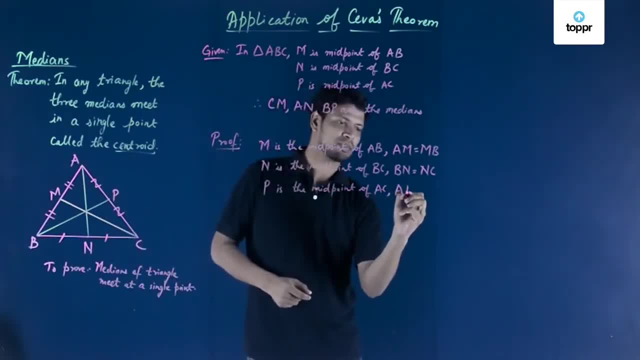 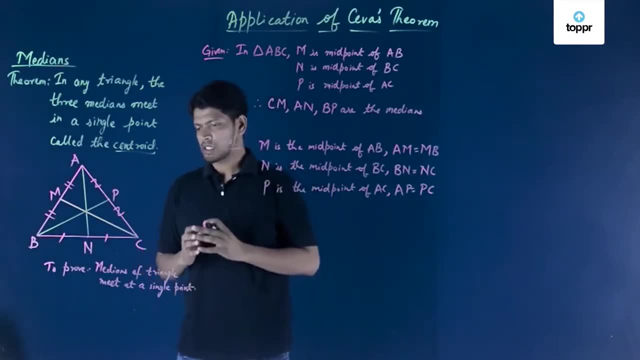 So we can say AP equal to PC. okay, So now, if for seeing that how this, we can prove by Siva's theorem what we will do. we will take the ratio of the available dimension or the length, and then we will. 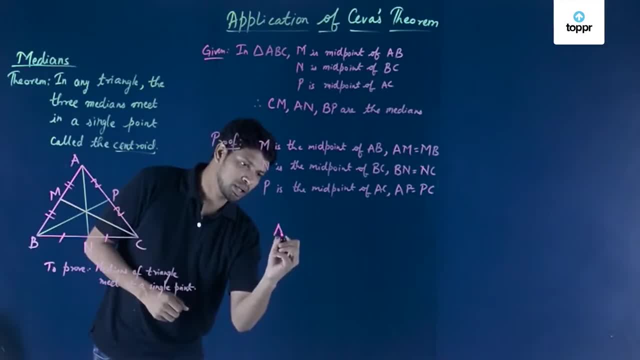 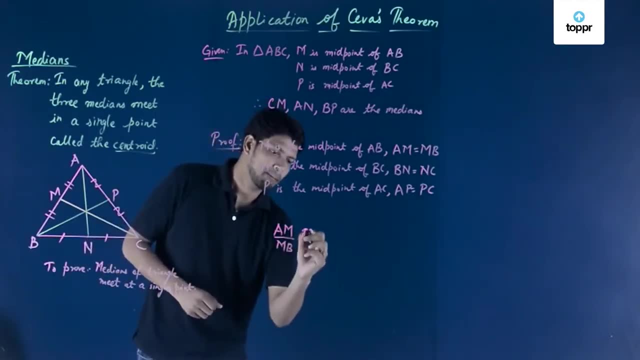 see what is the resultant. So if we take ratio of AM upon MB and we multiply that with BN upon NC, and that we multiply by AP upon PC, and we know that AM is equal to MB, So this will get cancelled and we 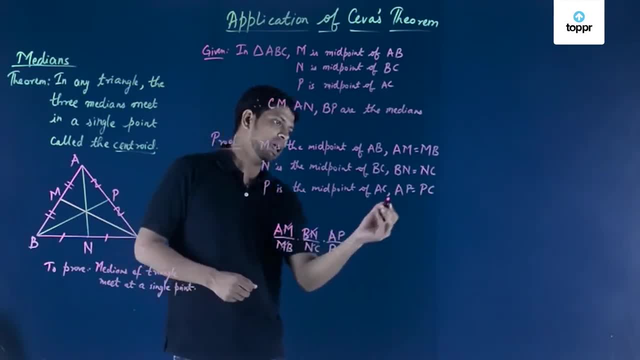 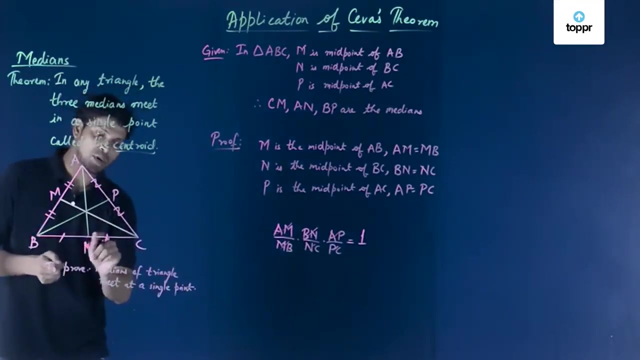 know, BN is equal to nC, So this will get cancelled. and AP is equal to PC, So this will get cancelled, and the resultant will be one. And this is same as in Siva's theorem, where it says that if AM upon MB into BN upon NC.